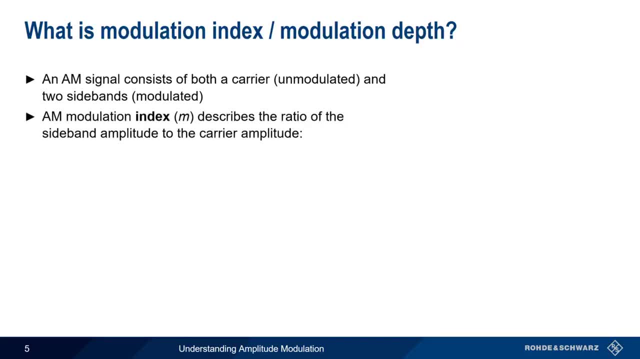 modulated sidebands. The AM modulation index, usually abbreviated with lowercase m, describes the ratio of the carrier and sideband amplitudes. In other words, m is the sideband amplitude divided by the carrier amplitude. We can measure the AM modulation index using two different types of instruments. We can 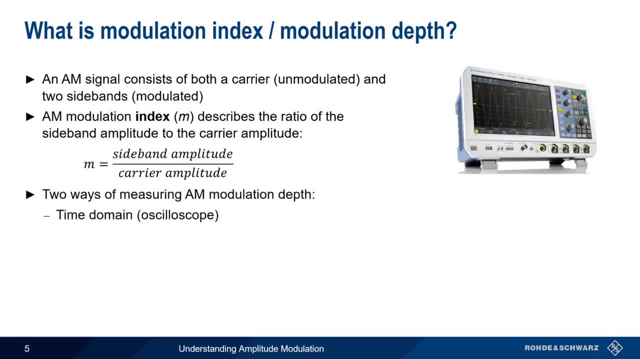 use an oscilloscope to measure modulation index in the time domain, or we can use a spectrum analyzer to measure modulation index in the frequency domain. We'll discuss both methods in this presentation. Note that you may also hear the expression AM- modulation depth. that is the modulation. 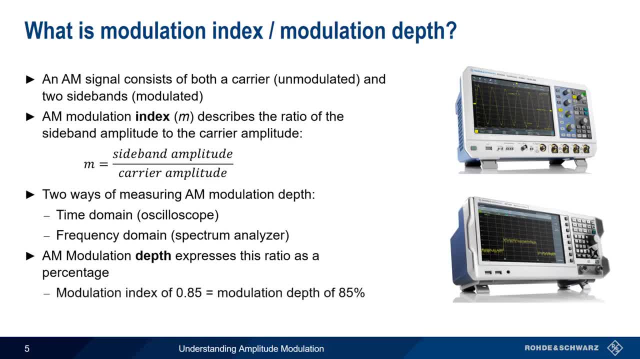 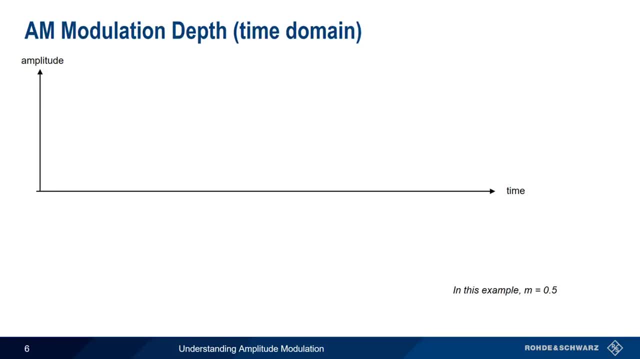 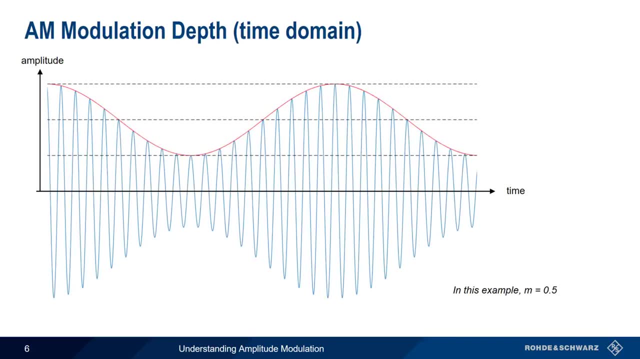 index expressed as a percentage. An AM modulation index of 0.85 is the same thing as an AM modulation depth of 85%. We'll start our explanation of AM modulation depth by looking at an AM signal. in the time domain, The amplitude of the carrier wave, the blue line, is changing over time. The 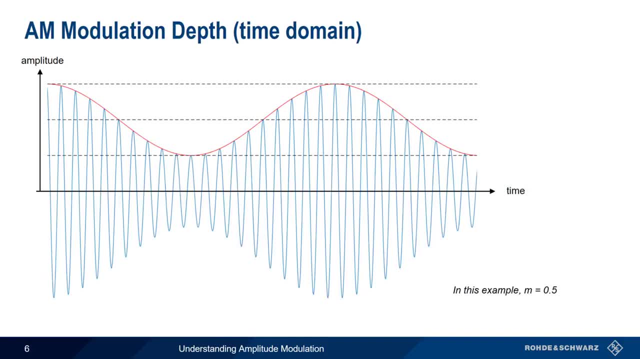 red line indicates what's usually called the envelope of the signal. The envelope has a maximum and minimum value. We'll designate the midpoint between these max and min values a sub c And we'll call the distance between the midpoint and the peaks a sub m. 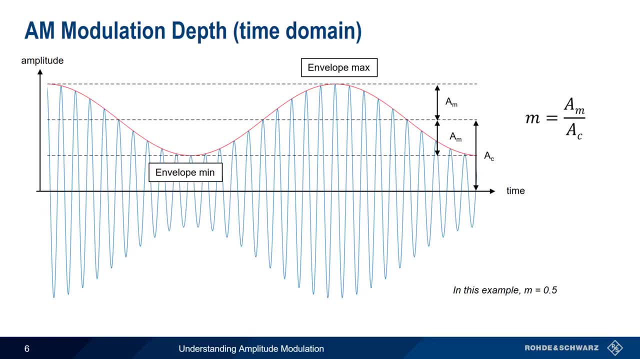 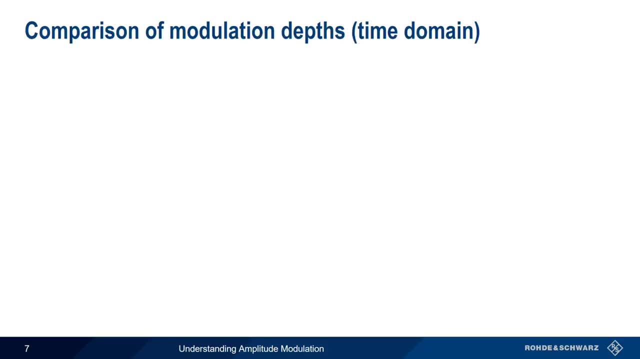 The modulation index m is simply a sub m divided by a sub c In the time domain. it's very easy to see why we sometimes refer to this as AM modulation depth. In the case of m equals 0.1, or 10% modulation depth, we can see that the envelope doesn't 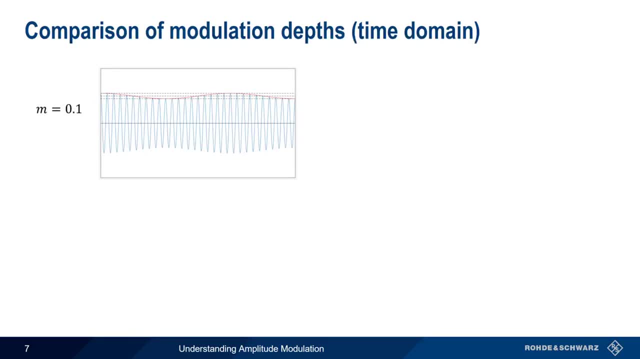 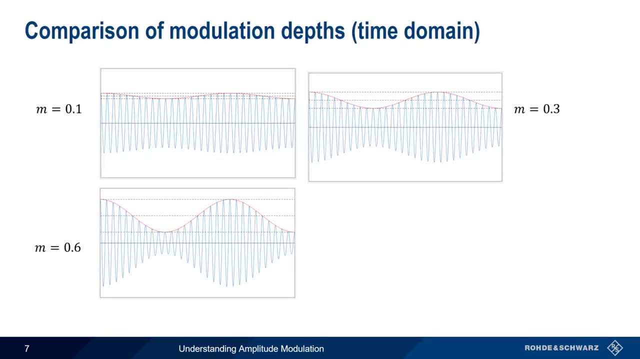 stray very far from the carrier. As the modulation index, or modulation depth, increases, the distance between the max and min envelope values increases, So we'll call this a modulation depth. The modulation index, or the peaks and troughs, also increases. When we get to m equals 0.9, or 90% modulation depth. 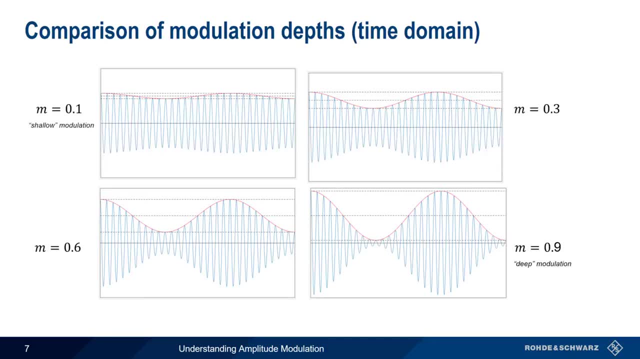 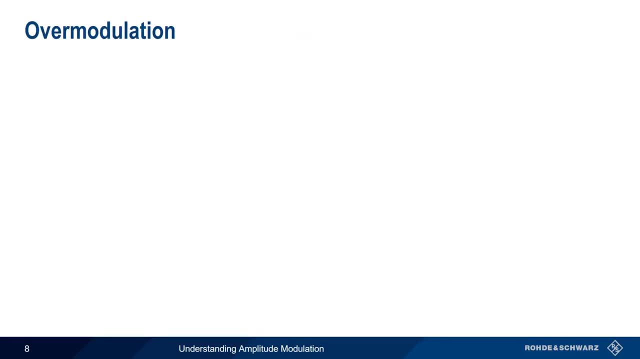 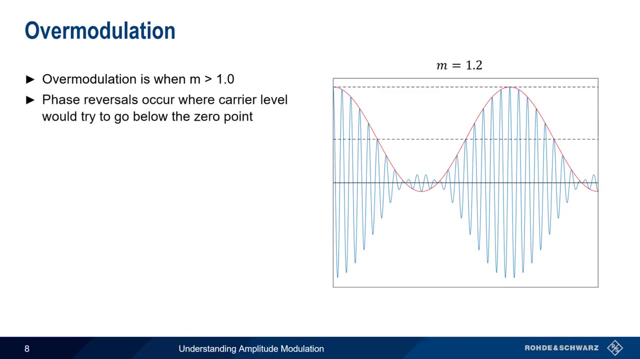 we have very deep valleys, or troughs, compared to the shallow valleys when modulation depth was only 10%. In case you were wondering, it is possible to have a modulation index greater than 1. This is called overmodulation. In an overmodulated signal, the carrier exhibits 180 degree phase. 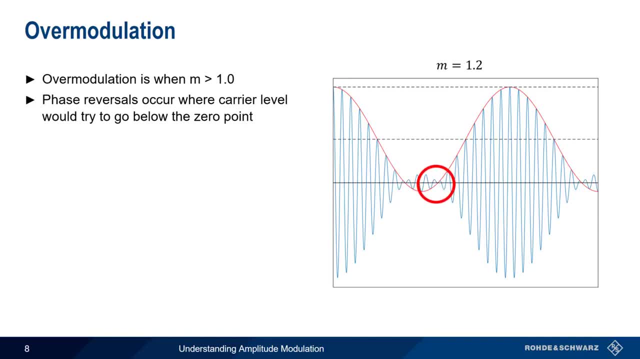 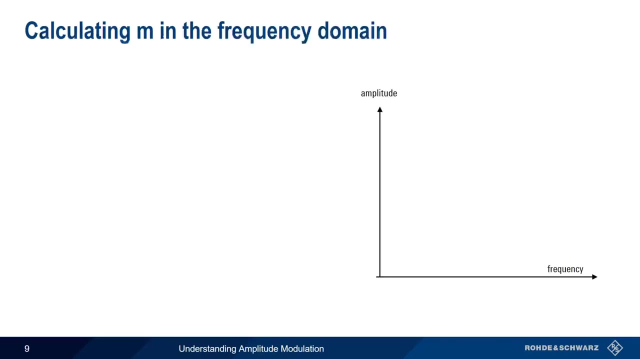 reversals where the envelope crosses the zero point. Overmodulation is undesirable because these phase reversals give ride to sidebands that can cause serious interference, sometimes referred to as splatter in nearby spectrum. As we saw a few moments ago, an AM-modulated signal in the frequency domain consists of an. 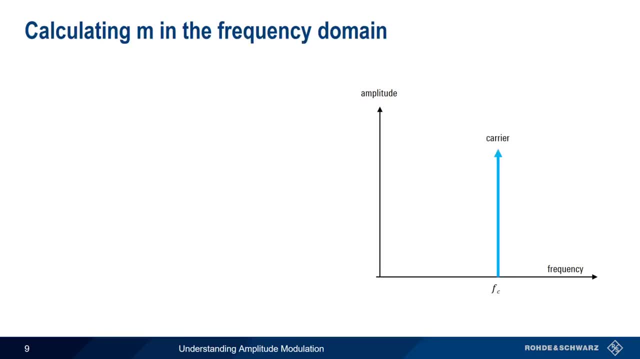 unmodulated carrier and two modulated sidebands, One upper sideband and one lower sideband. The väger aggressive modulator and call IN-M years ago presented more than 50 different performance outputs on both sides of those caps. sonra-mersателяe feel very high in modulations. when one visualized again, the frequency gets up by aструкhat and by certain levels with or with mult venues in of those caps, As you can see the properties of an AM-modulated audio signal, sometimes under multiple modes and versus inner demand. in other words, you maybe will saying 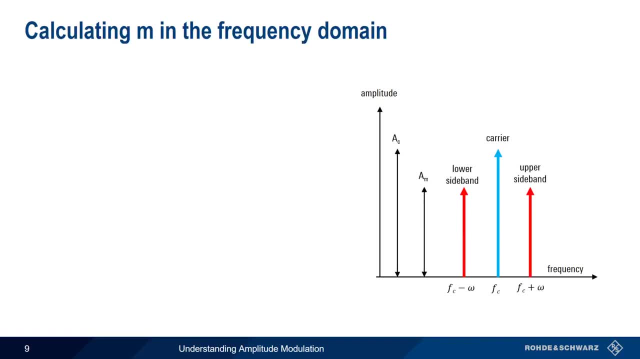 The values a sub c and a sub m from our time domain discussion are also shown here. Modulation depth m can be calculated in the frequency domain by measuring the difference in amplitude between the carrier and the sidebands. This difference, n, is normally negative and expressed in dBc. 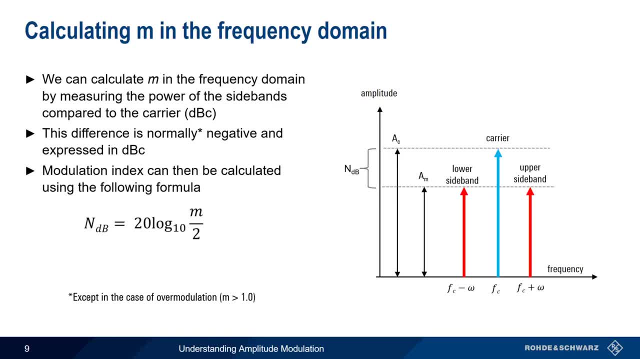 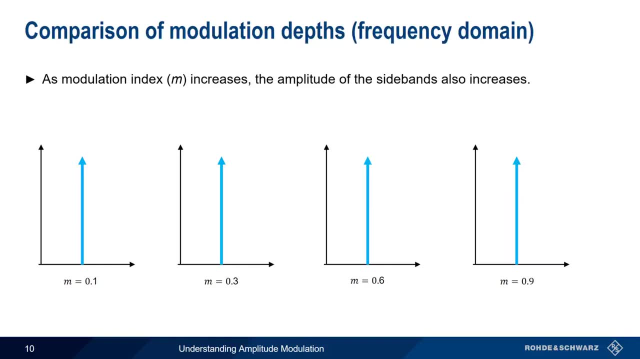 We can then calculate modulation index using a simple formula. As we increase the modulation index, m, the amplitude of the sidebands also increases, And n, the difference between the carrier and the sidebands therefore decreases. It's important to note that carrier amplitude is unaffected by modulation depth. 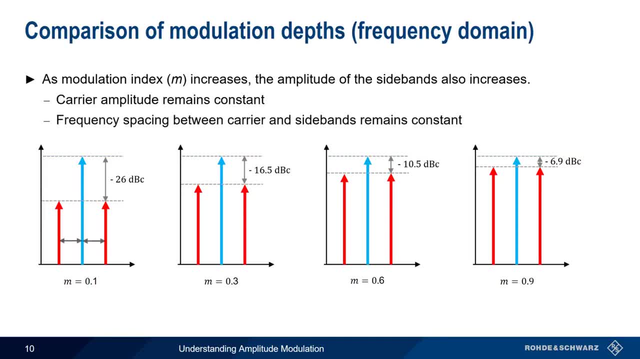 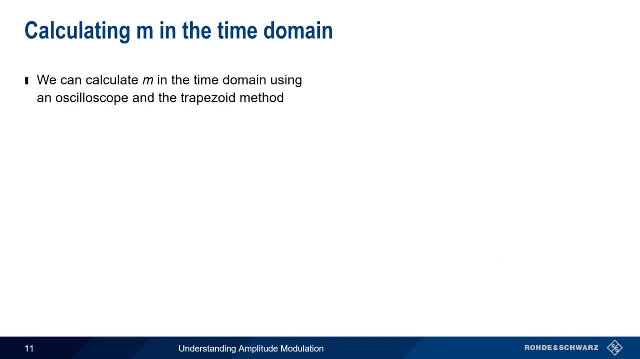 Note also that the frequency spacing or distance between the carrier and the sidebands does not depend on modulation depth In the time domain. we can calculate the modulation index m using an oscilloscope and the so-called trapezoid method. 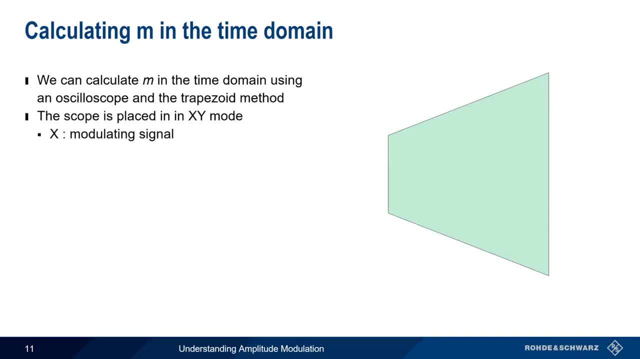 This is done by placing the scope in x-y mode, with x being the low-frequency modulating signal and y being the amodulated RF signal. This causes a trapezoid to appear on the scope display, and modulation index is calculated using the lengths of the two vertical edges, a and b, as well as a sub c. 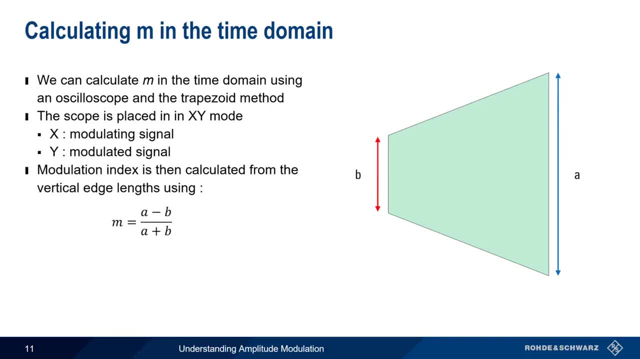 In the time domain. we can calculate the modulation index m using an oscilloscope and the so-called trapezoid method. This is done by placing the scope in x-y mode, with x being the low-frequency modulating signal and y being the amodulated RF signal. This causes a trapezoid to appear on the scope display, and modulation index is calculated using the lengths of the two vertical edges, a and b, as well as a sub c. Scopes generally don't have an automatic measurement functionality for amodulation.